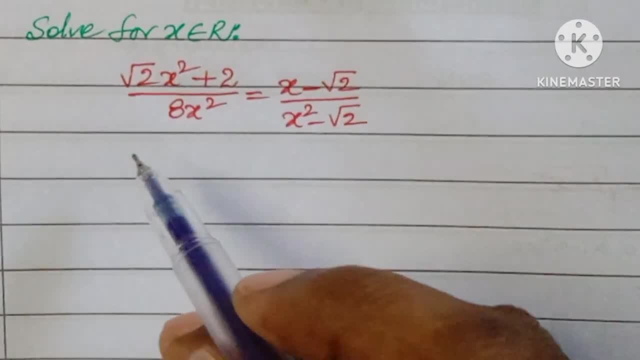 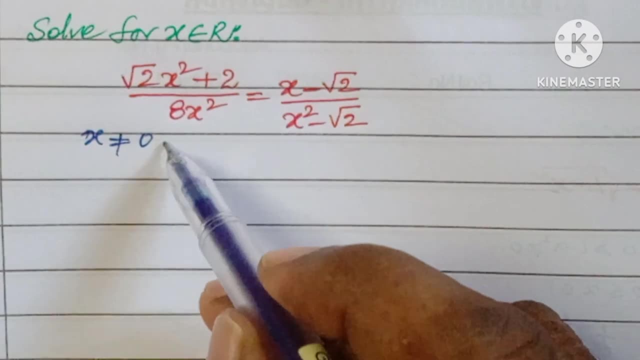 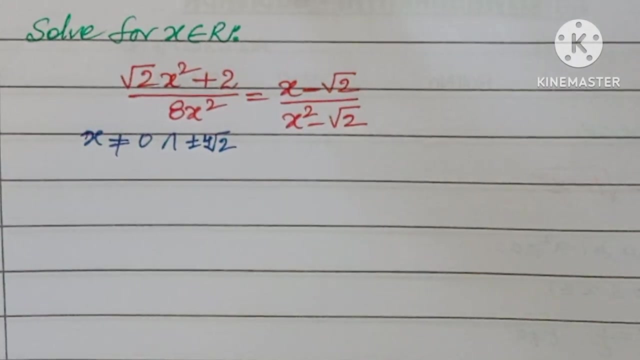 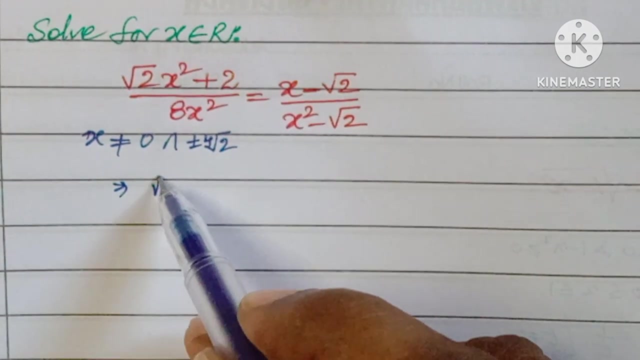 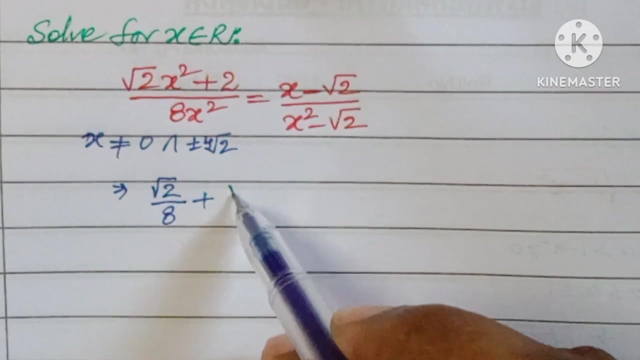 Now how to solve this. So here, first of all, by observation: x value is not equal to 0.. And x value is not equal to plus or minus 4 root 2.. So here, first of all, we will divide with x square denominator root 2 by 8 plus root 2, whole square by 8 x square. 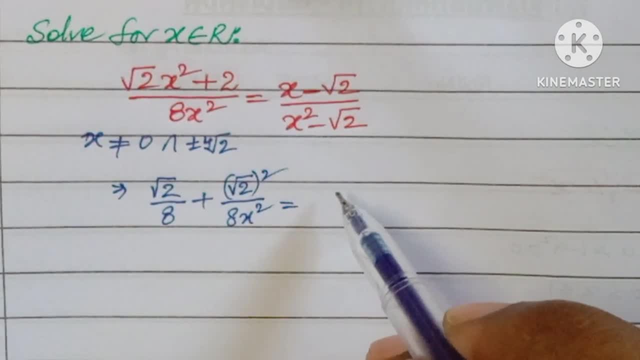 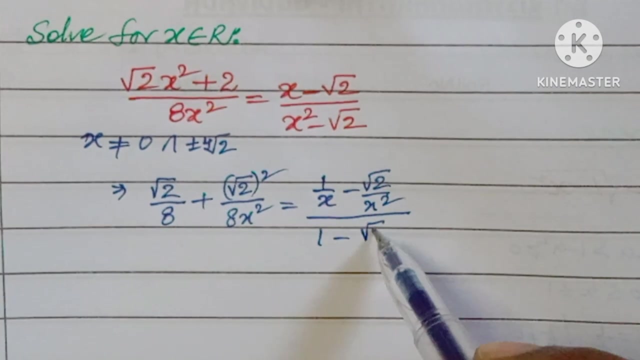 So the other side we will take, we will divide by x square Here, 1 by x minus root, 2 whole square by 8 x square, 1 minus root, 2 by x square, And the denominator will be 1 minus root, 2 over x square. 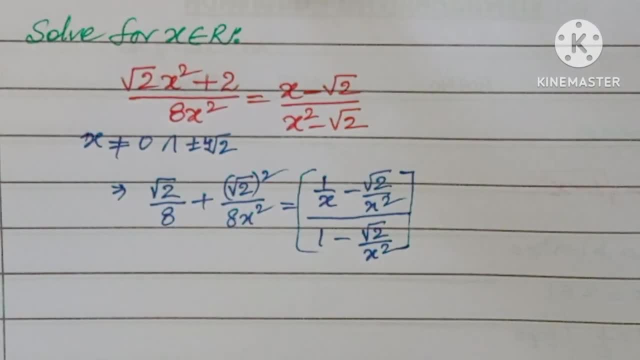 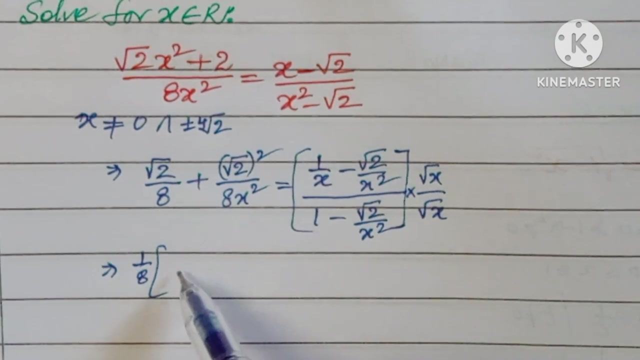 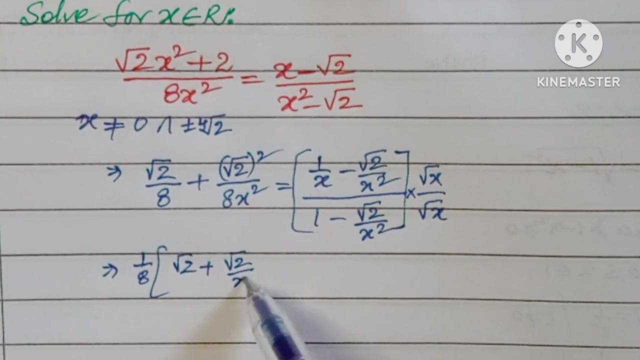 So dividing both side with x square. So here multiply with root x in numerator and root x in denominator. So here I am taking 1 by 8 common in LHS, 1 by 8 into root 2 plus minus root. 2 by x, whole square. 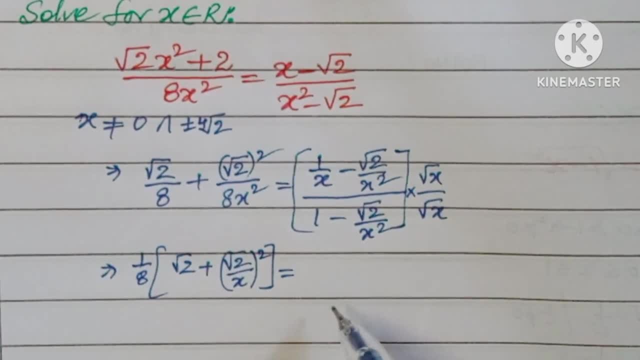 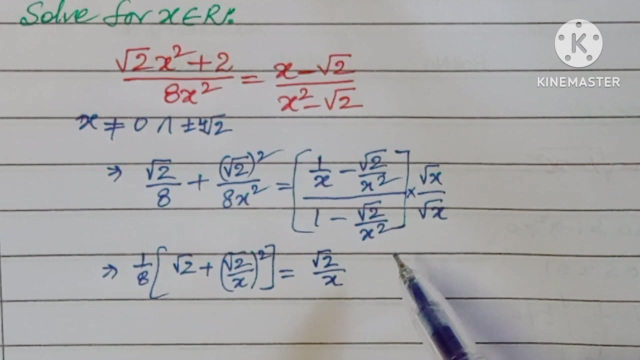 So this is equal to if you multiply with root x. So here what we will get: root 2 by x, root 2 by x. I am sorry, multiplying with root x Minus root 2 by x, whole square. 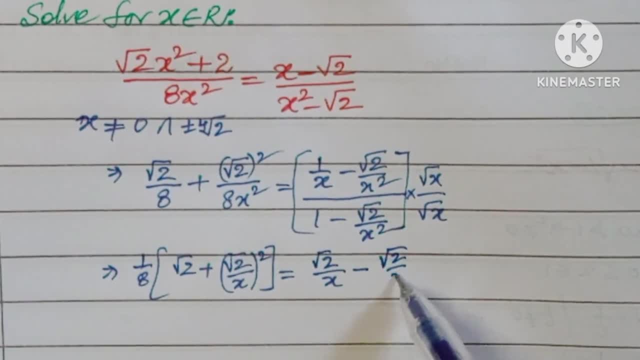 So this is equal to if you multiply with root x. so here what we will get minus root 2 over x whole square. by here we will get root 2 minus root 2 over x whole square. So here minus root 2 by x whole square. 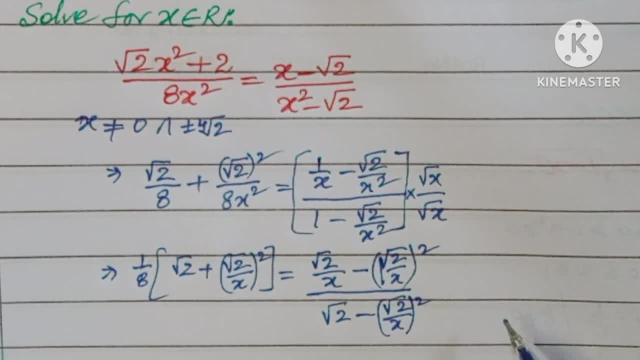 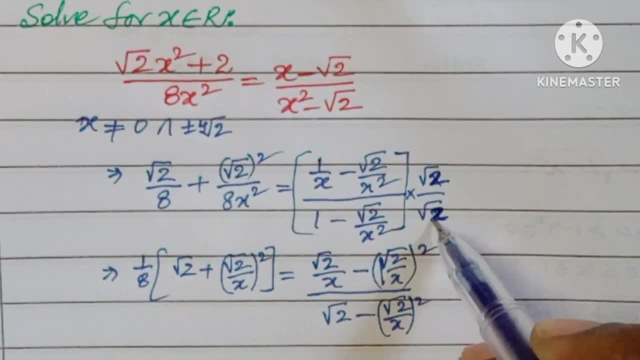 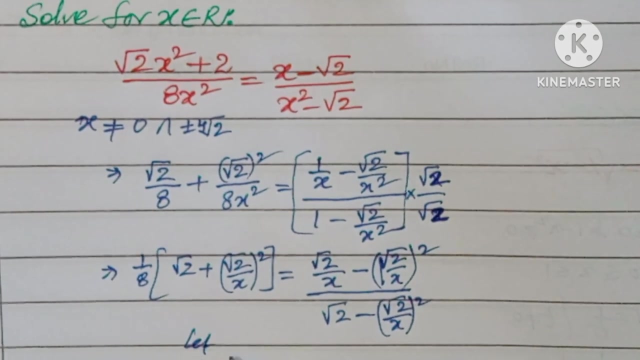 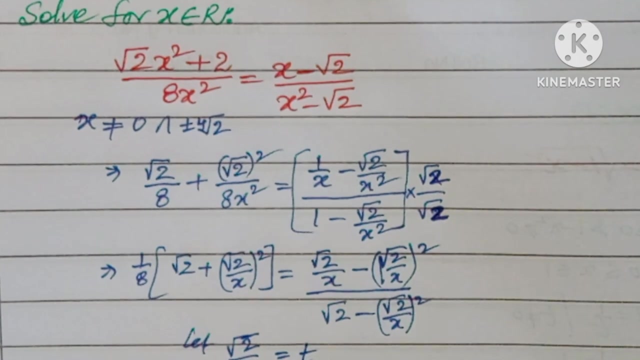 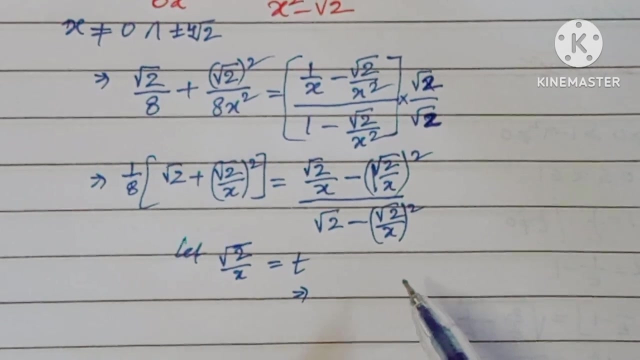 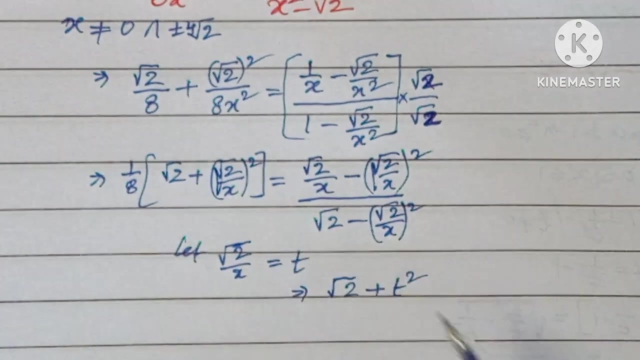 So here minus root 2 over x whole square. So here Multiplying with root 2, here both in numerator and denominator, Now let us take root 2 over x is equal to t. Now the equation will change here: root 2 plus t square, root 2 over x whole square is equal to. 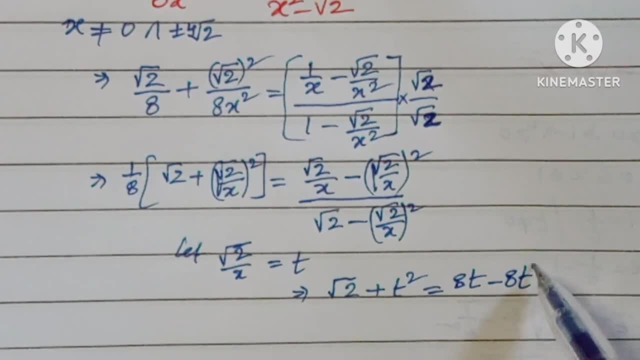 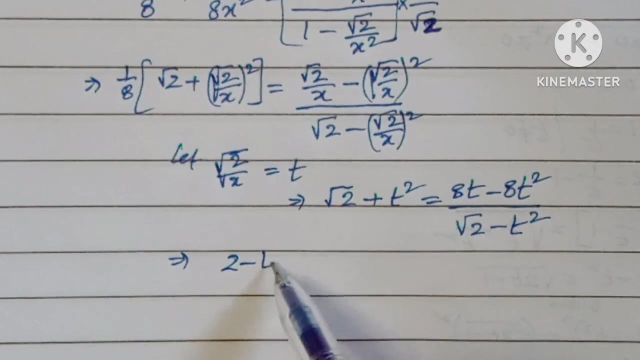 8t minus 8t square root, 2 over x. x as t root, 2 minus t square. Now, if you cross, multiply this: 2 minus t to the power of 4 is equal to 8 t minus 8 t square. Now here you will get t to the power of 4, sending all. 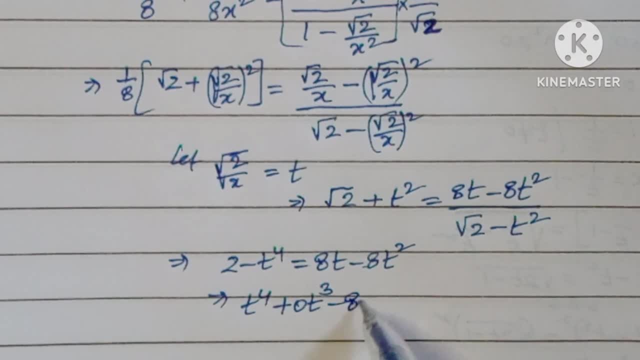 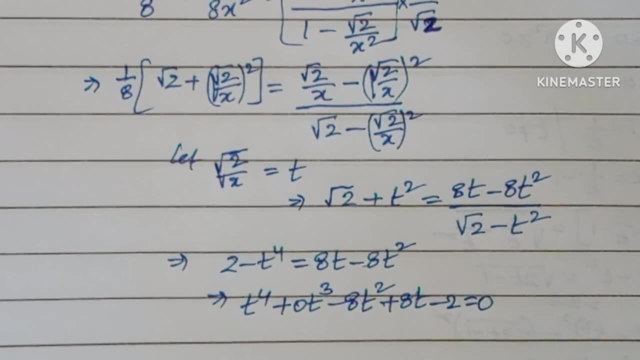 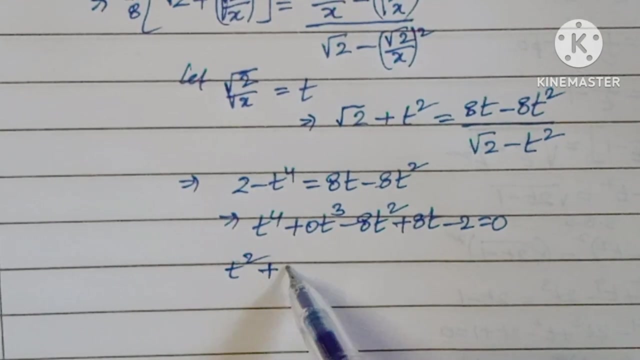 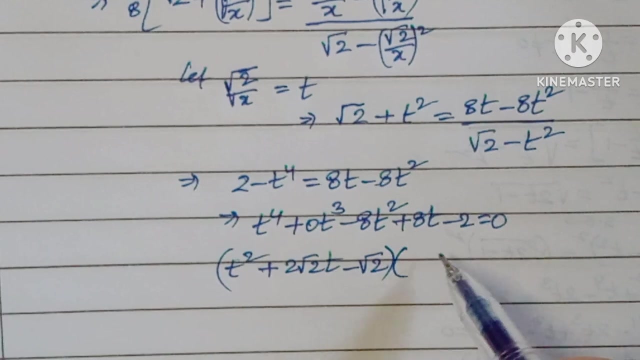 the terms to one side as 0 t cube minus 8. t square plus 8. t minus 2 equal to 0.. Now here we are going to do factors: t square plus 2, root 2, t minus root 2 into t square. 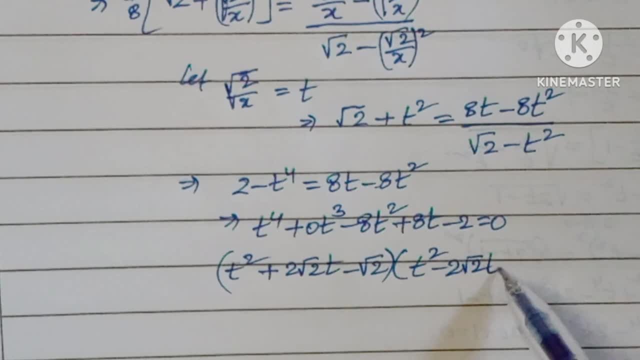 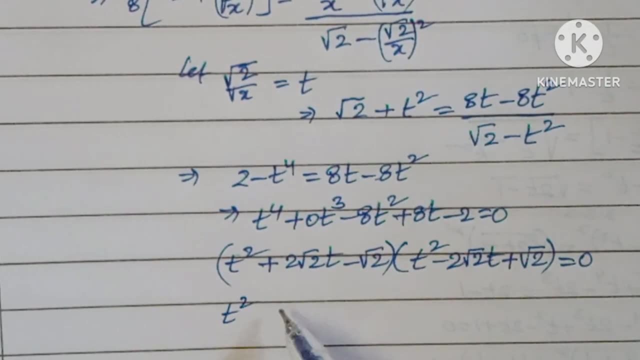 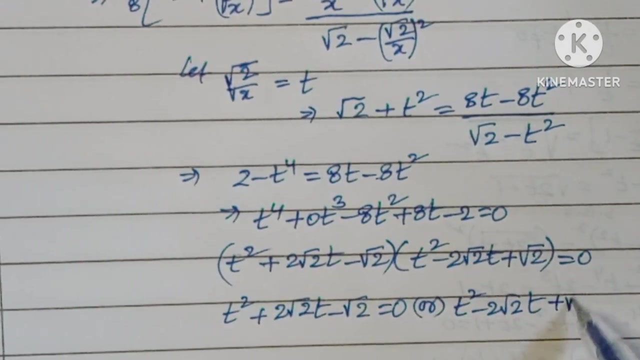 minus 2 root 2.. plus root 2 is equal to 0. now T square plus 2 root 2. T minus root 2 equal to 0. or T square minus 2 root 2. T plus root 2 equal to 0. now, here you have to find the. 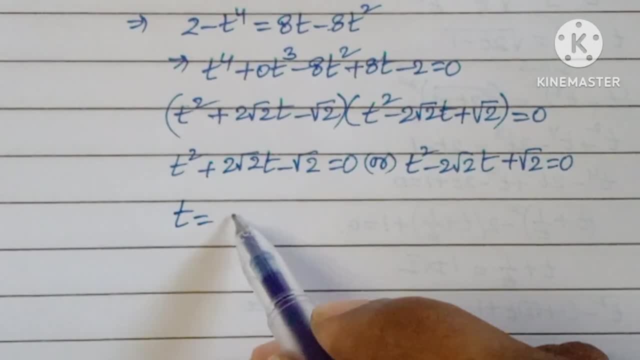 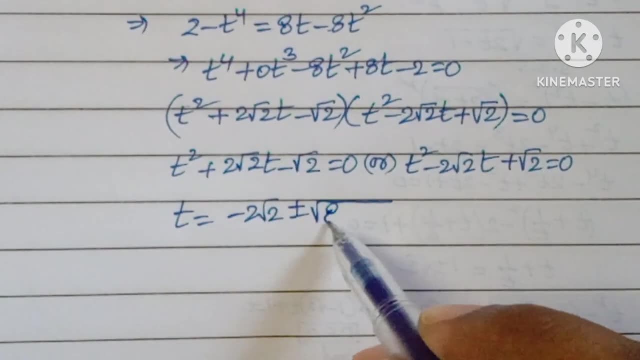 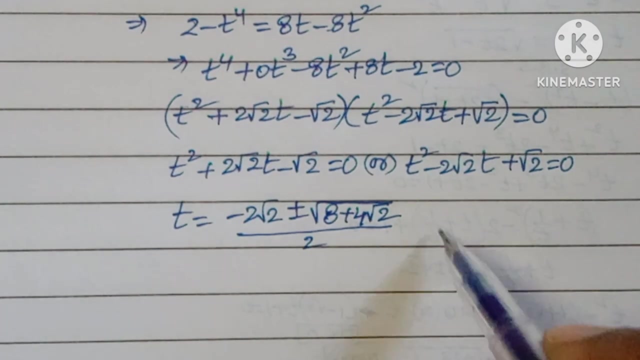 value of T. so T is equal to minus 2 root 2 plus or minus square root of 8 plus 4. root 2 over 2. okay, T is equal to 2 root 2 plus or minus root of 8 minus 4. root 2 over 2: okay. 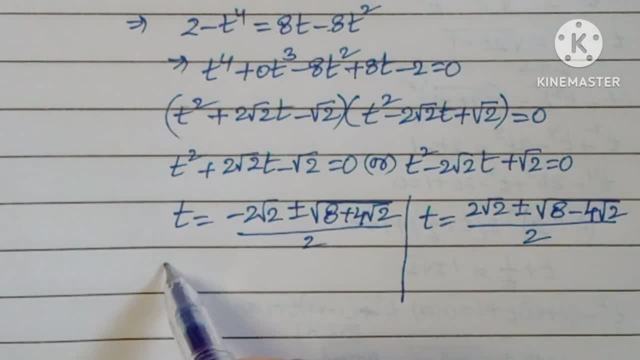 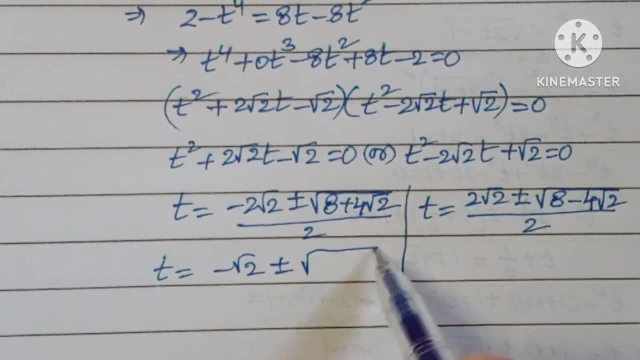 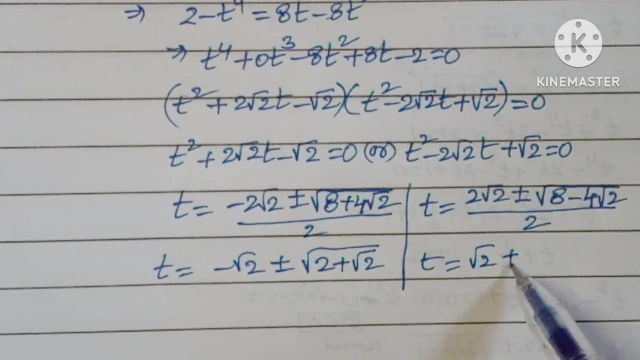 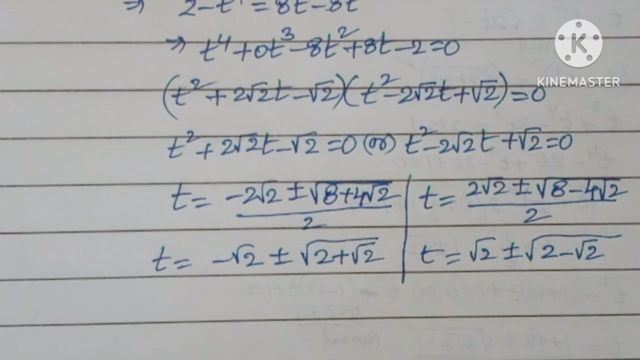 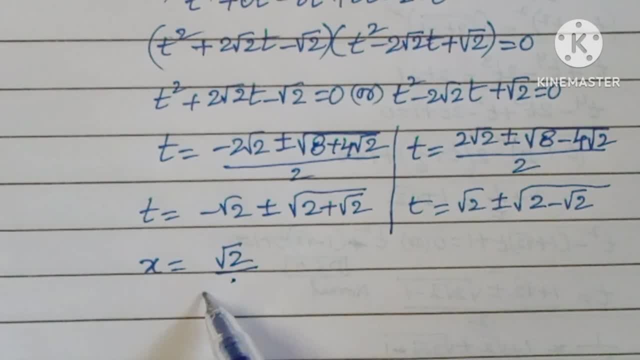 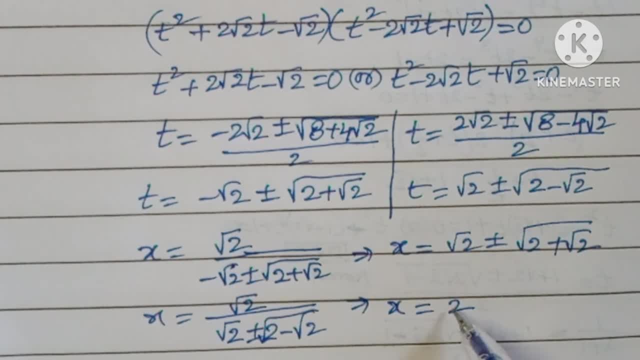 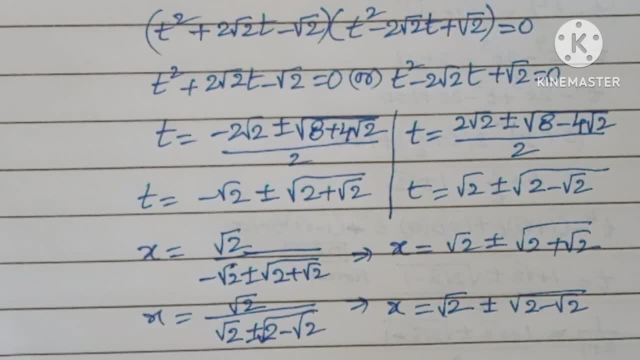